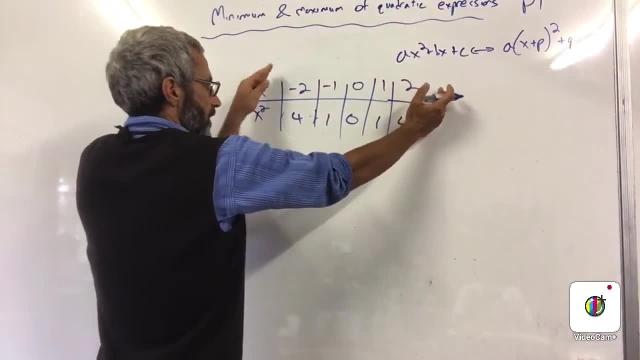 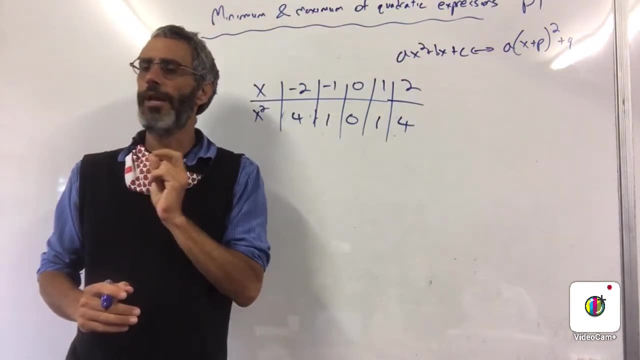 Okay. So basically, if I carry it on, minus 3, I'll get 9.. Plus 3, I'll get 9.. We notice that. okay, let's put it this way: Is there a maximum for this quadratic expression? Is there a maximum? 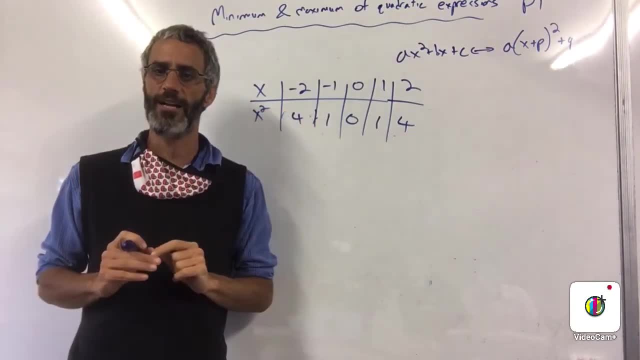 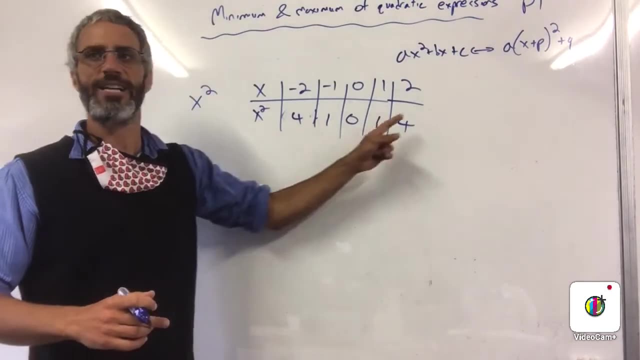 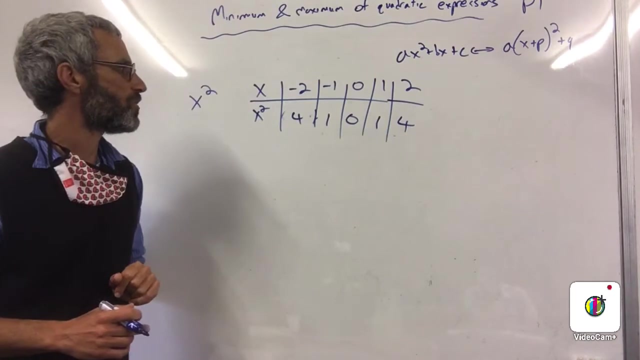 Is there a certain value that you're never going to get higher than this? No, As I increase x, I'm going to get higher and higher numbers. But is there a minimum? Yes, There is a minimum. There is a minimum. What is the minimum? What was the smallest number that you can get x squared to be equal to? 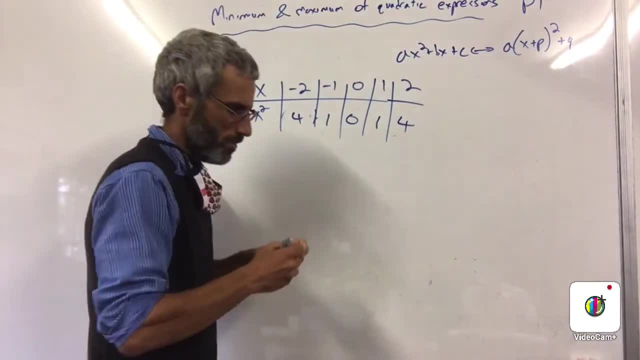 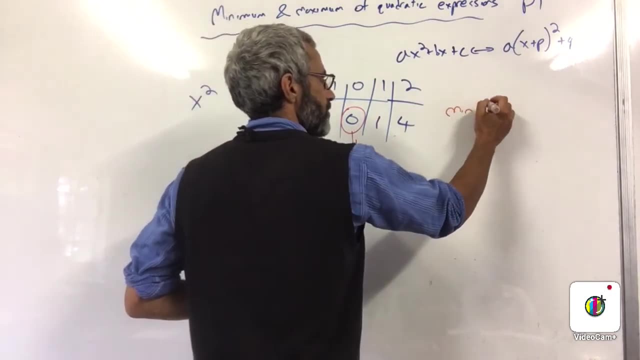 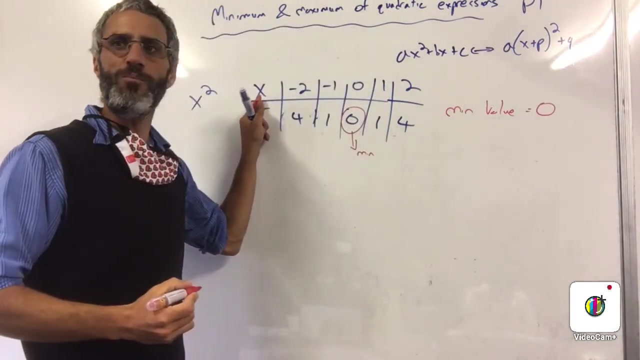 0.. 0.. 0.. Okay, So this is your minimum Minimum. okay, Minimum value, right? Minimum value equal 0.. What does x have to be to give you the minimum value? What is the x value? 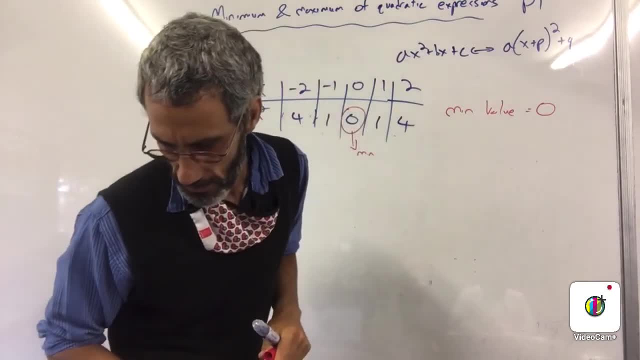 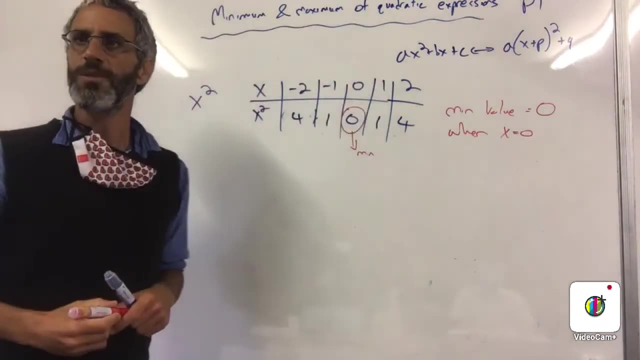 0.. 0.. 0.. Okay, So I just want to say it the same way. Okay, So I'll write it when x equals 0.. That's how I'm going to write it. Okay, It's kind of obvious, right. 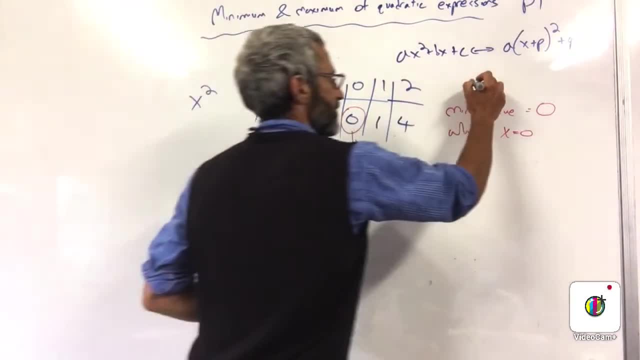 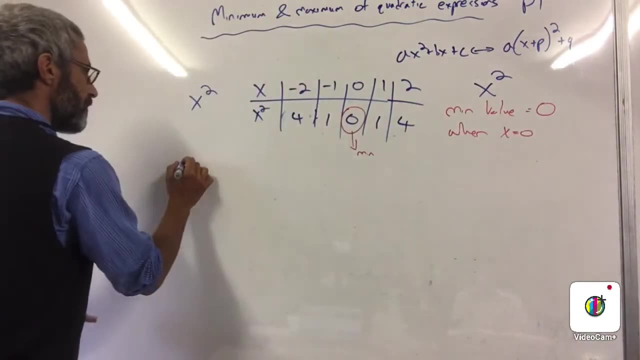 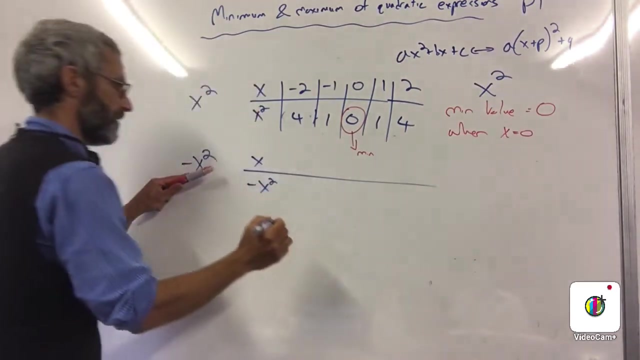 Now let's do the same thing. Okay, I'm going to write that. So the minimum value of x squared is equal 0, and that happens when x equals 0.. Let's do the same thing for minus x squared. Okay, So I'm going to have x and minus x squared. This is a different quadratic expression, Okay. 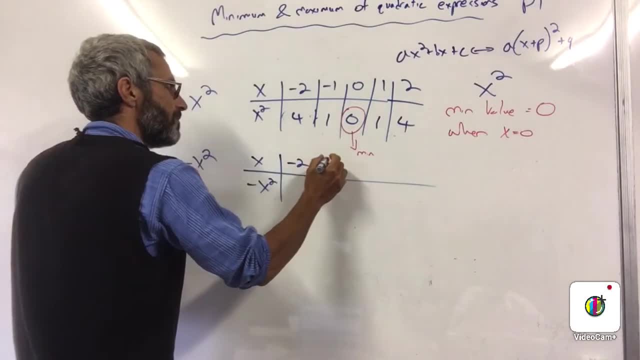 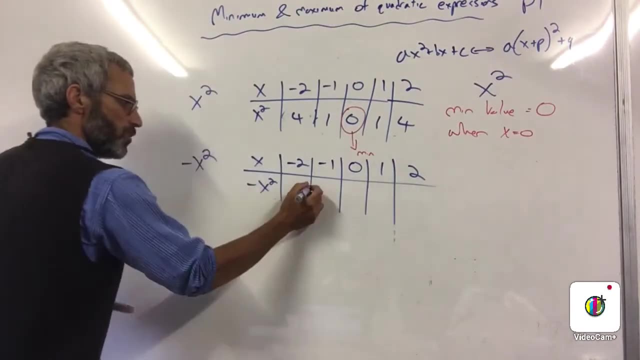 I'll just time it by minus 1.. Let's do the same thing: Minus 2, minus 1, 0, 1, 2.. Okay, Eventually, hopefully, I don't have to do this, but in the beginning we do that, Okay. 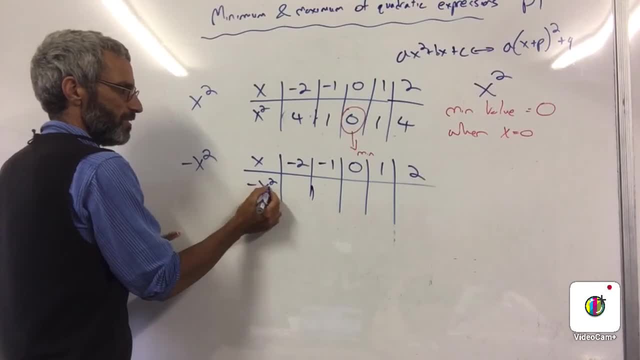 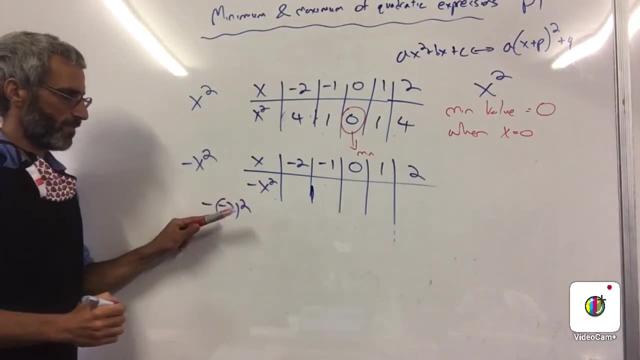 So what will be? minus minus 2 squared? Okay, Minus minus 2 squared. How much is that? Minus 4., Minus 4., Minus 4.. Minus minus 1 squared, Minus 1.. 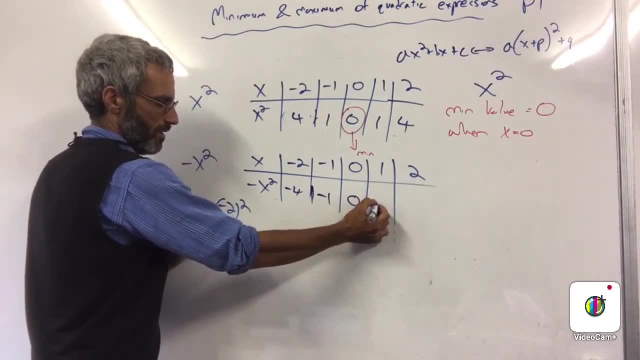 Zero Zero, Minus 1.. Minus 1.. Yeah, Minus 1 squared, Minus 1.. Minus 1: squared is minus 1, and this one, Minus 4.. Minus 4.. 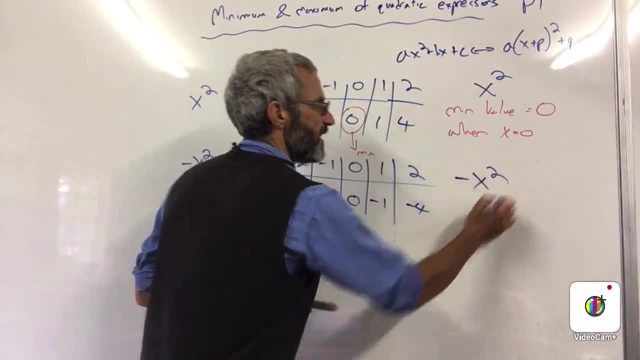 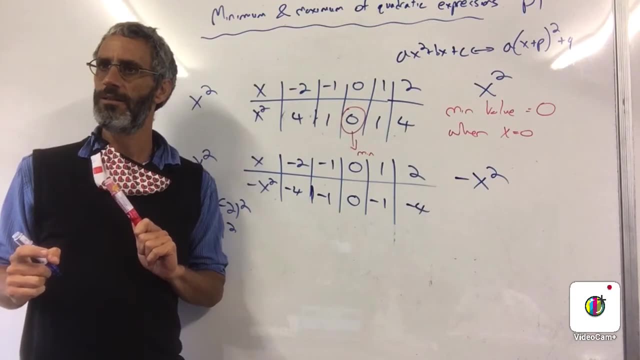 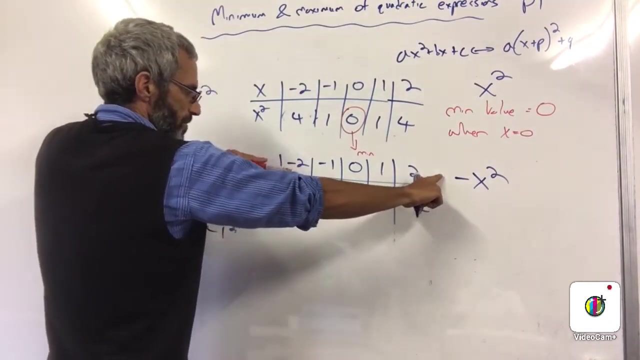 Okay, All right. So this expression minus x squared, does it have the minimum or maximum? now, Minimum, It has a maximum, It has a maximum. See, as I carry on with 3, and minus 3, and 4, and minus 4,, the numbers will get smaller and smaller and smaller, right? 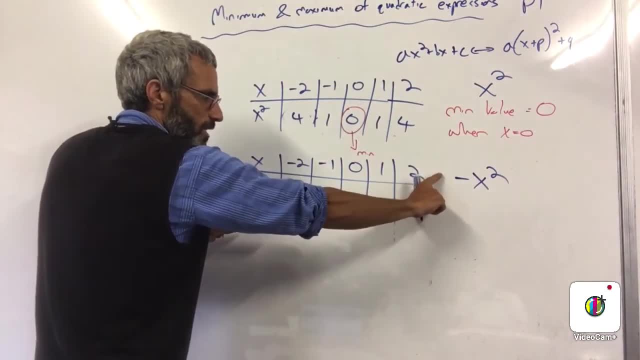 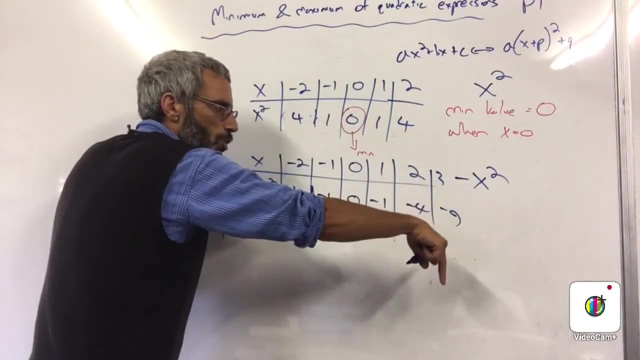 The next number will be minus 9,. right When x equals 3.. Right When x equals 3, the next one will be minus 9.. Minus 3 will also give you minus 9, so the numbers are getting smaller and smaller and smaller. 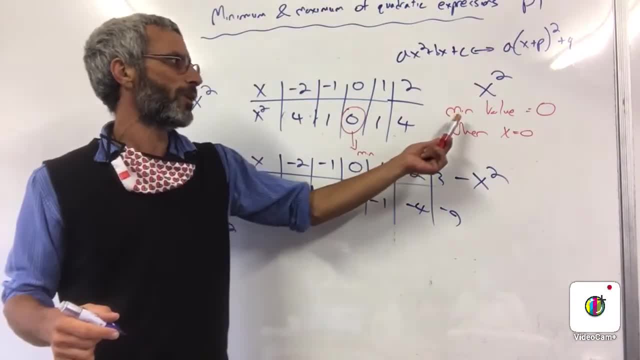 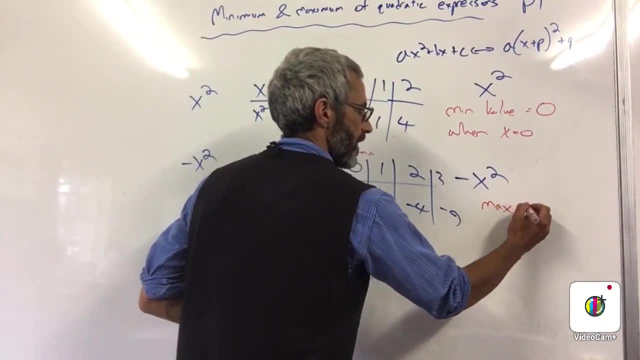 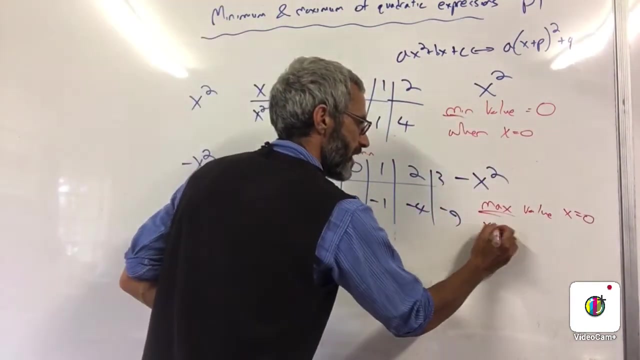 Okay, If numbers are getting smaller and smaller and smaller, that means that there is no minimum, but there is a maximum. Okay, What is the maximum value now? Zero. Maximum value is again zero. It's a maximum, It's not a minimum. And for which x does that happen? 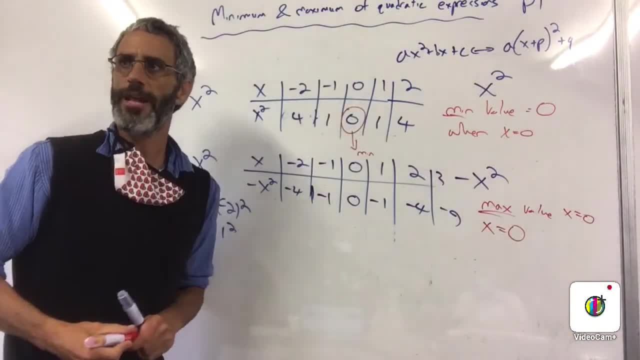 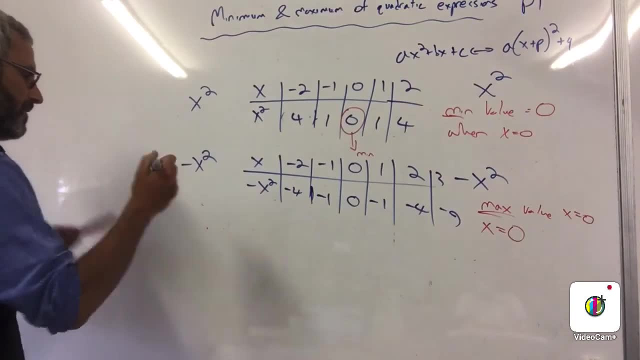 Zero, Zero, Zero. We happy with that. I'm just going to pause here. Okay, We're going to carry on and maybe now I'm going try not to draw this table. Let's see, Let's say I have x squared plus two. 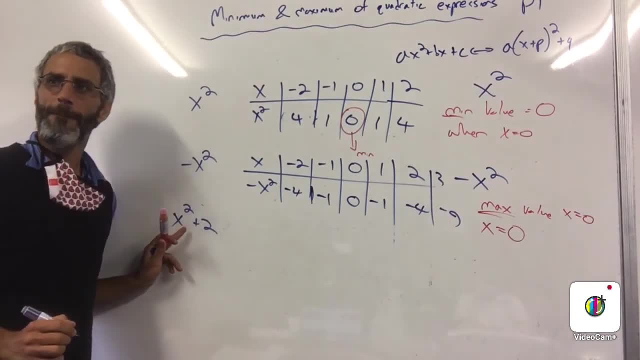 Let's ask you first of all, does it going to have a maximum or a minimum value? Minimum, It's going to be a minimum value. Can you see it? or should I draw this table? Let's draw the table. Let's just do one more time. 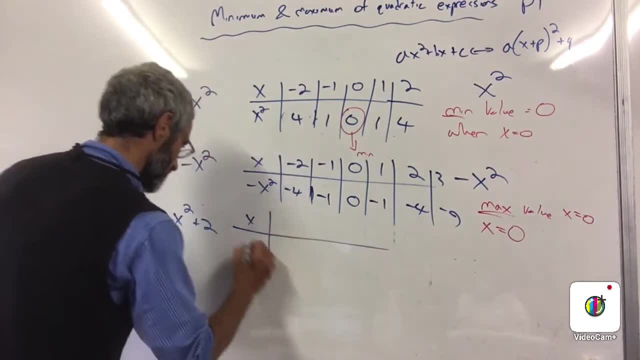 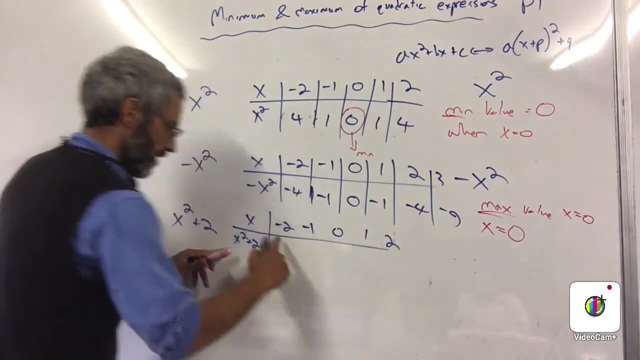 Okay, So I've got x, and now I'm drawing x squared plus 2.. Okay, Let's just do the same: Minus 1,, 0,, 1, and 2.. If I put minus 2 squared plus 2,, what will I get? 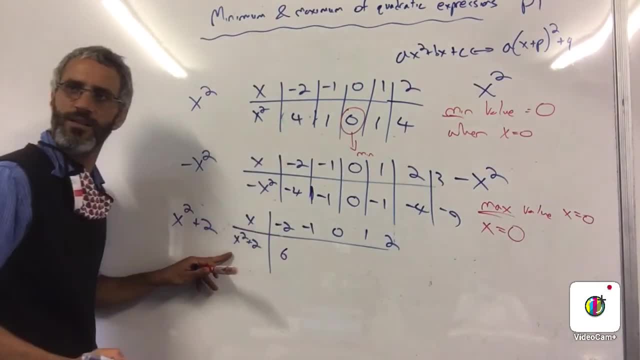 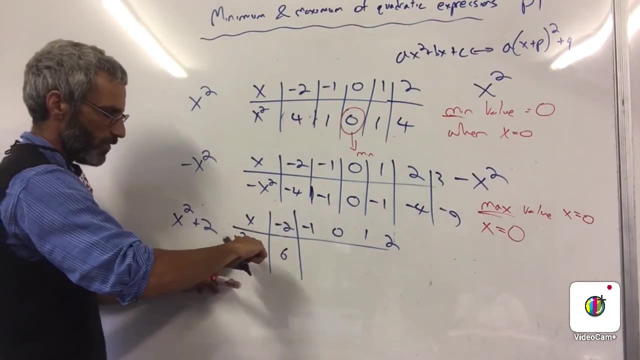 Well, I had 4 plus 2, that would be 6, right, Okay, I'm just putting: minus 2 squared 4 plus 2 is 6.. Minus 1 squared plus 2 is going to be 3, I think. 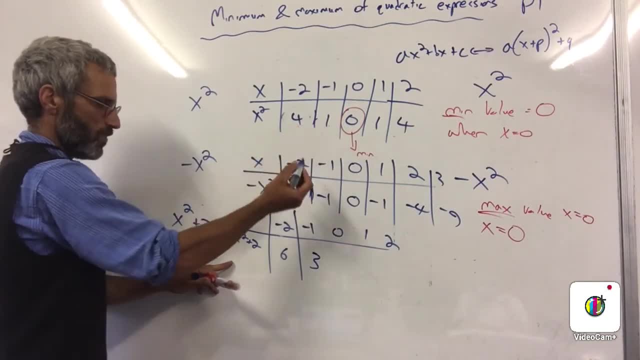 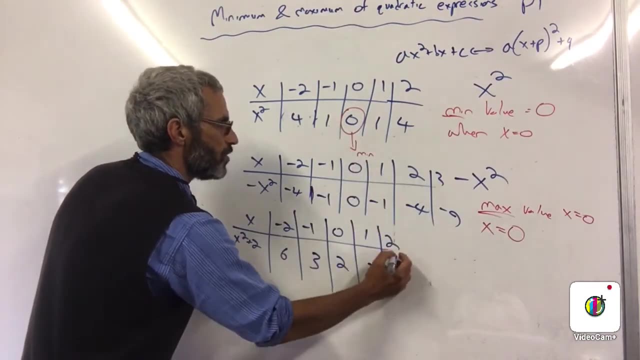 Yeah, I'm just adding. I'm really adding 2 to each one of these numbers, right? This one is going to be 2. And then this one is going to be 3, and this one is going to be 6.. 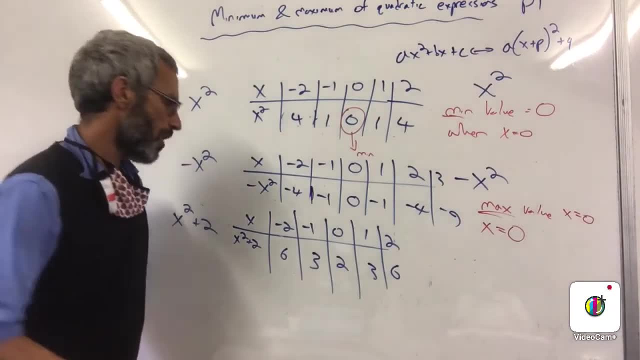 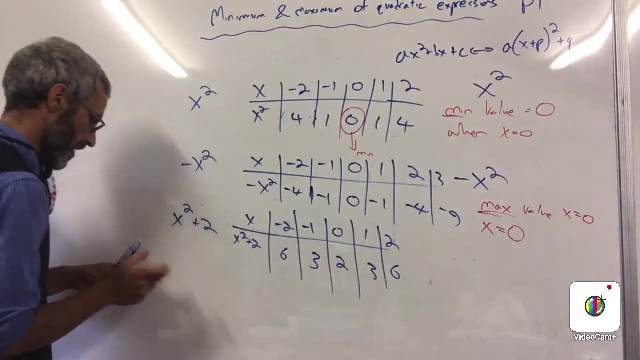 Okay. So what do I have here? I'll write it down here. Is it a maximum or a minimum? It's going to be a minimum, okay. Okay So, minimum, Minimum value. what will be the minimum value? It's 2.. 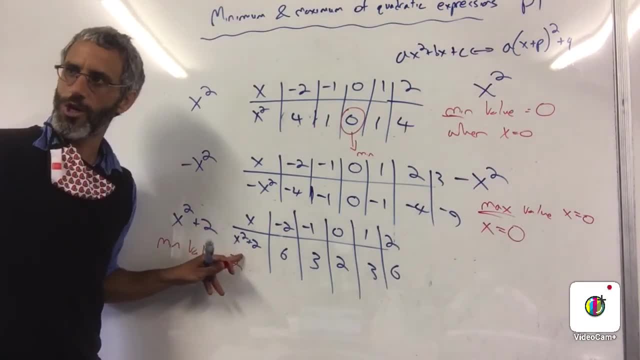 It's 2, okay, Really, when we learn about function, we call this a vertical shift. Remember, a vertical shift moves it up. These are actually parabolas, Okay, Anyway. Alright, minimum value is 2.. For which x does that happen? 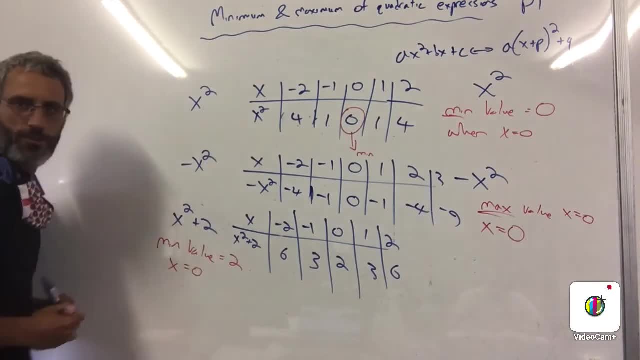 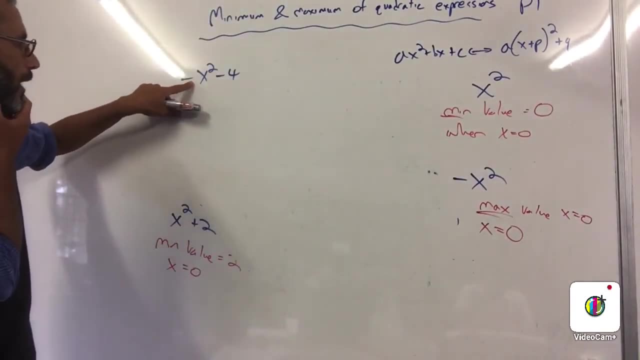 Zero. Okay, I'm just going to pause and make some space here. Now we're moving on to another quadratic. This is a quadratic expression, so it has a minus before the x squared and a minus 4.. Let's try and really do it now, without the table, okay. 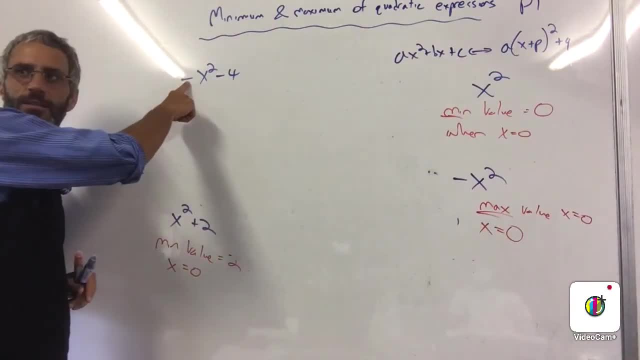 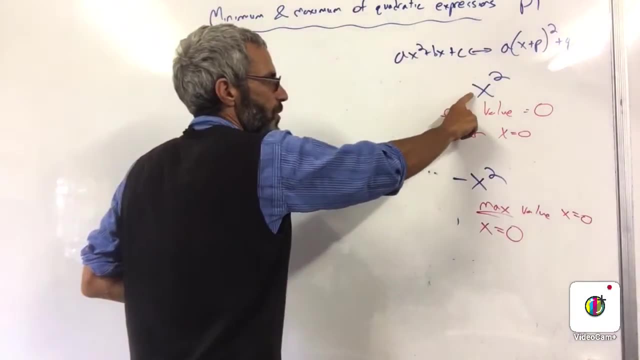 First of all, the fact that we've got a minus here that should be able by now to see, to know if it's a maximum or minimum. Let's just look at all the ones we had here. When we had a positive before the x squared, that means we had a minimum. 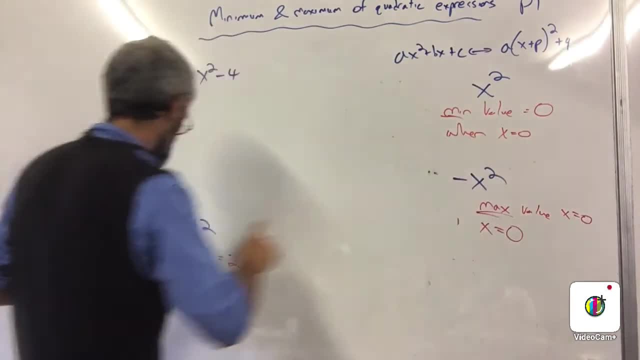 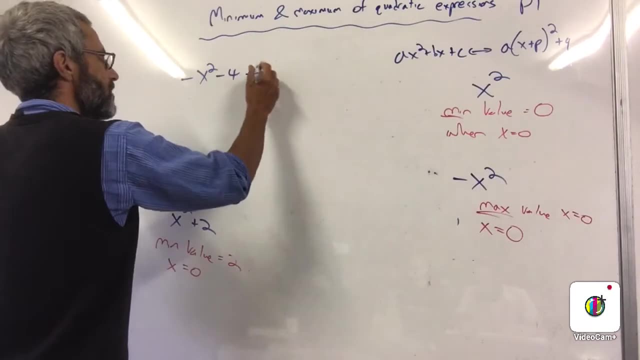 When we had a negative, it was a maximum. When it was a positive, it was a minimum. So what do you reckon this is? What do you reckon that will be? It will be a maximum. okay, It's going to be. let's do it anyway, okay. 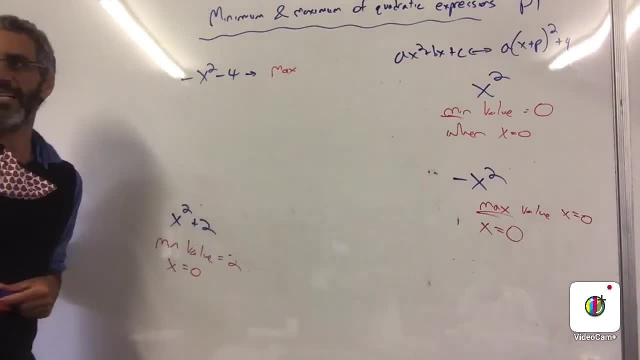 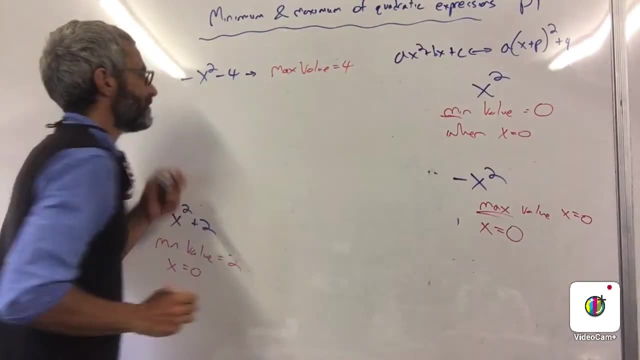 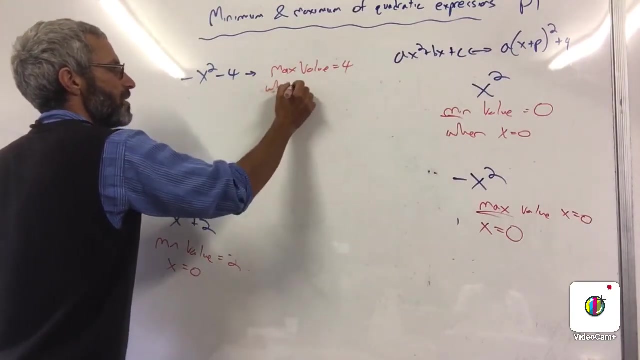 A maximum value. What will be the maximum value? Zero, It will be negative 4,. okay, And let's try and understand that. Before we try and understand that, for which x will it be this value, When x is equal to what? 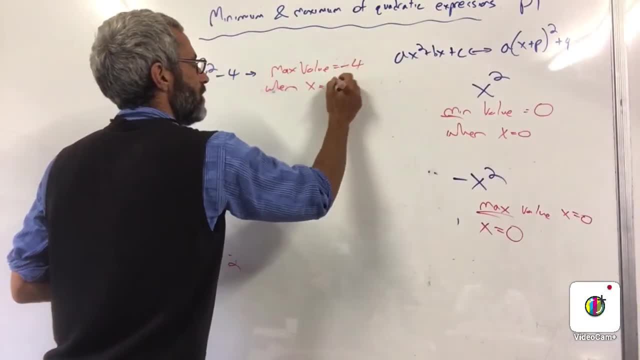 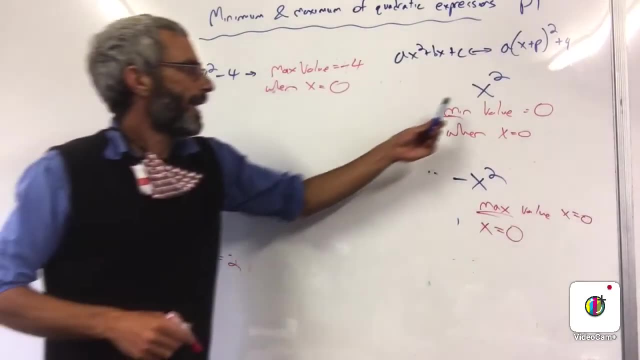 Zero. That should be minus 4.. Okay, Absolutely Okay. So what's happening here? Let's try and think about what we've done here. x squared- because I've got squared- is always a positive number, right Okay? 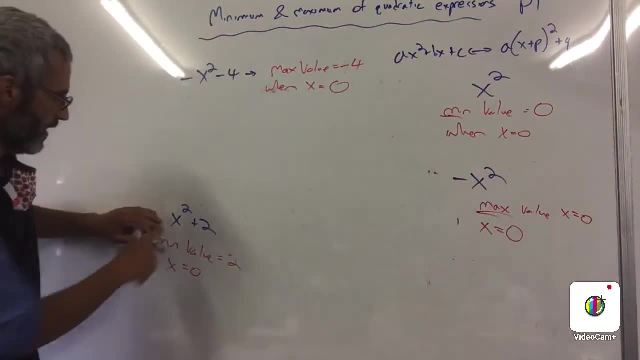 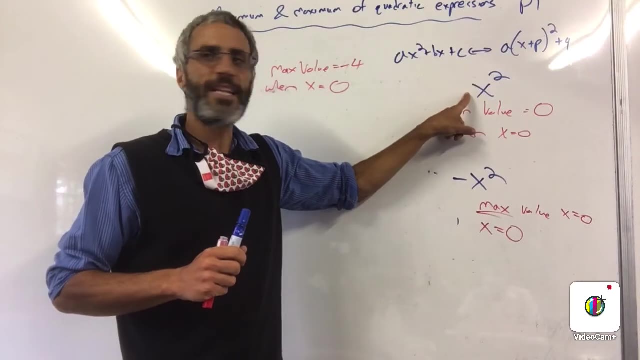 x squared is positive, x squared is a positive, x squared is a positive. So it's always. it's never going to be negative, But the smallest it can be. what's the smallest it can be? x squared- Zero. Okay. 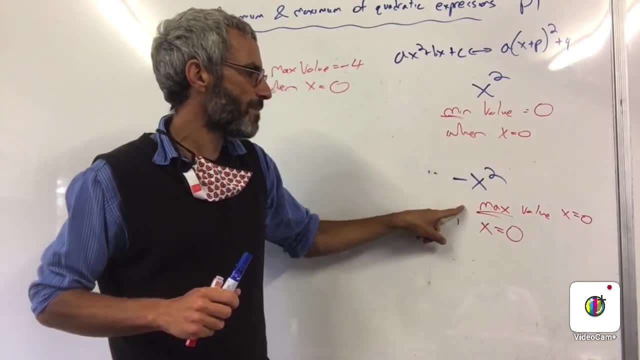 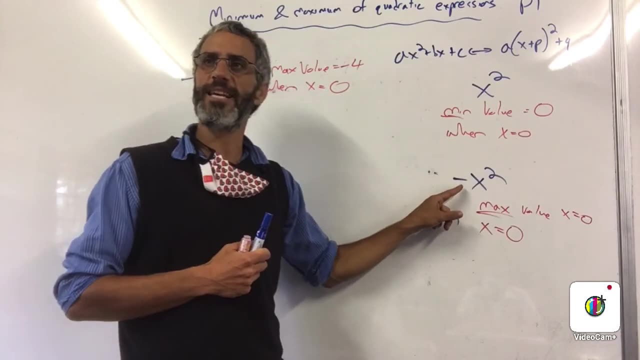 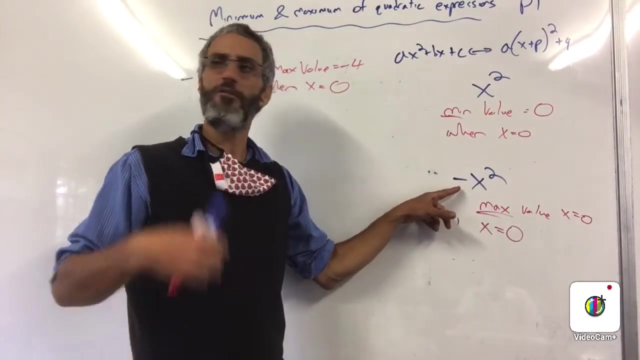 So that's why the minimum here is zero. Now, why is it maximum when I have that negative number? Because x squared is always positive. That means minus x squared is always negative. So if it's always negative, okay, that means we have a maximum here. 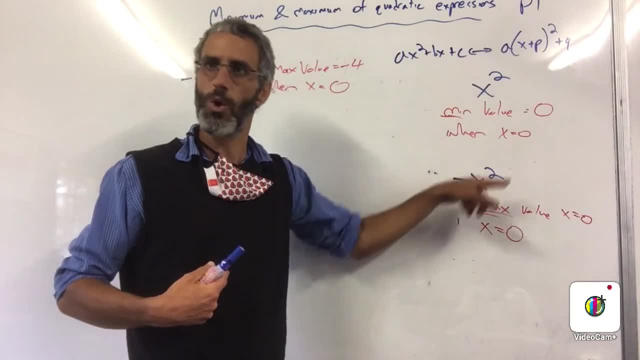 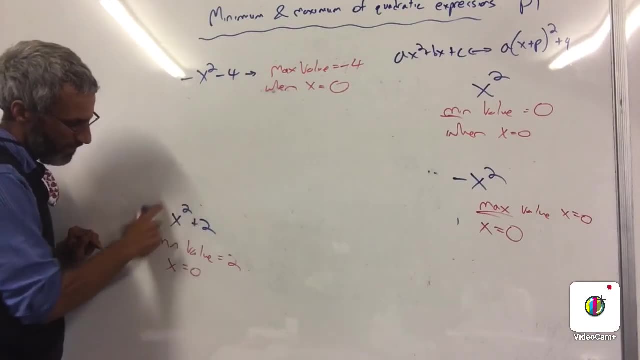 What is the maximum here? when x is equal to zero? So this whole thing, the value of zero, is the maximum. Okay, The same thing here, right, Because this is always positive. The lowest it can be is x equal when x is zero. this whole thing is zero. 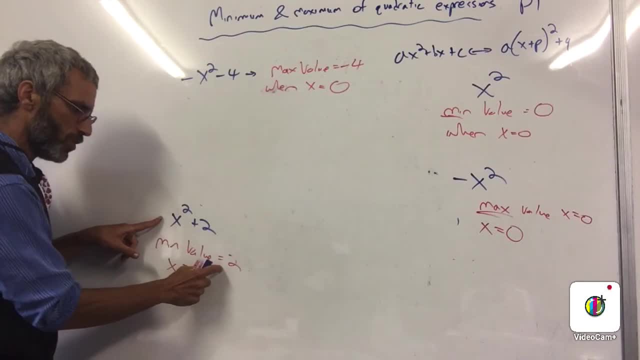 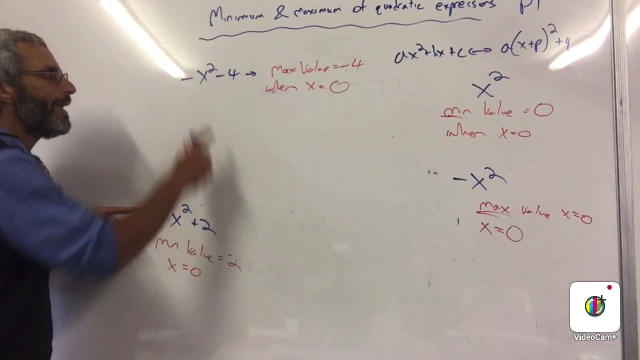 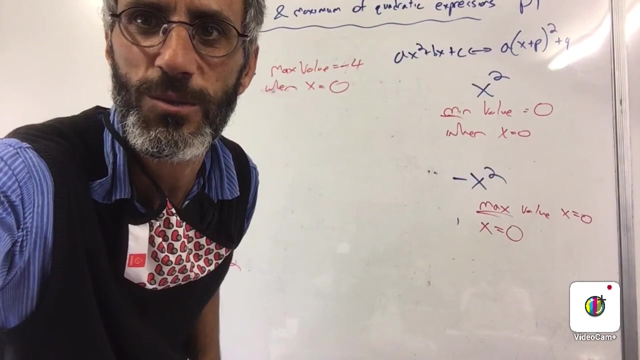 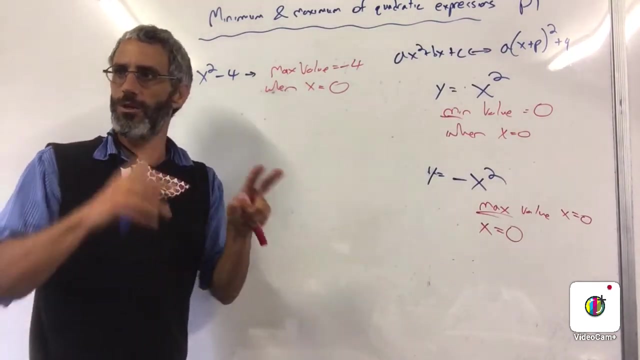 Now, because I have plus two, the max, the minimum value, is going to be plus two. Um, if you're happy with that, Oh yeah, Is it working? Yes, I think it was So far. all these kind of expressions we've looked at last year when we drew these parabolas. 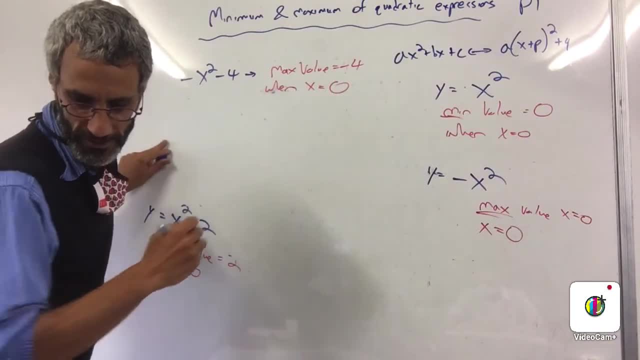 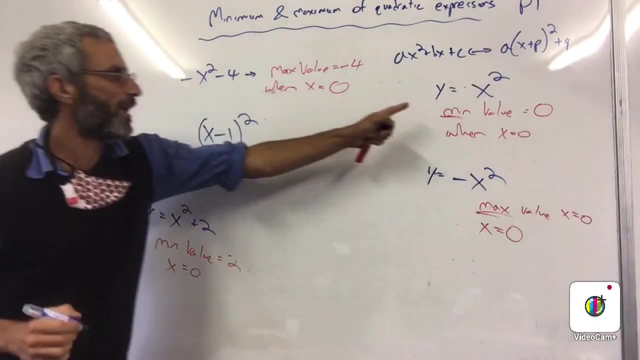 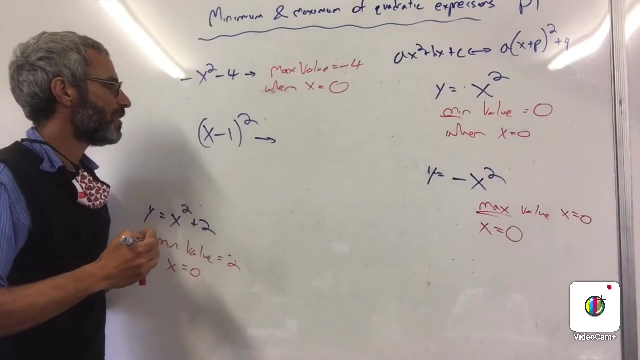 Okay, But now we're going to have something a little bit different, So let's go with that x minus one squared, So it's not x squared, x minus one squared. First of all, from what we've learned now, will it have a minimum or a maximum? 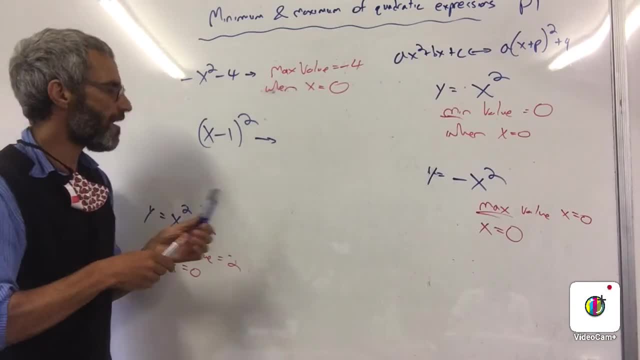 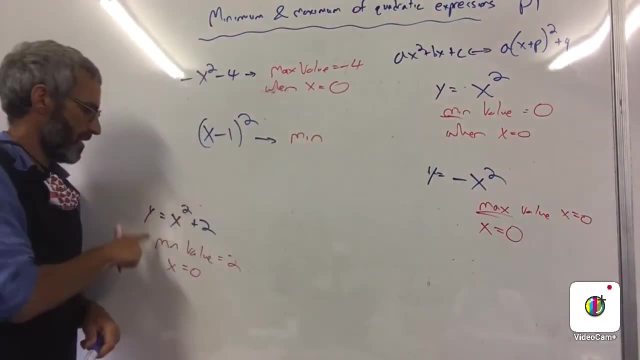 It's going to have a minimum. It's going to have a minimum Because I don't have a negative. it's positive on this side, like here, like here, it's going to have a minimum. Yeah, Because all of this is positive, right. 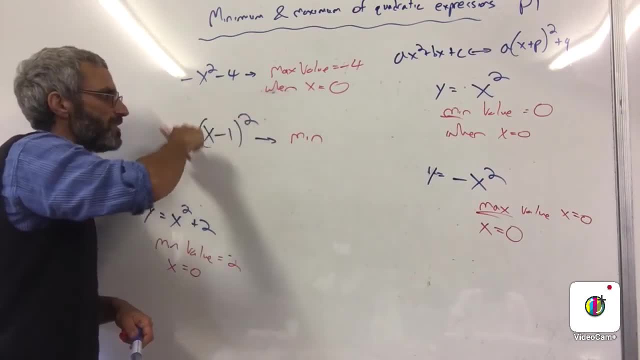 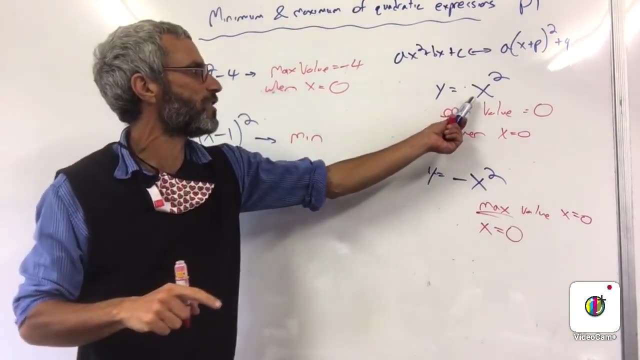 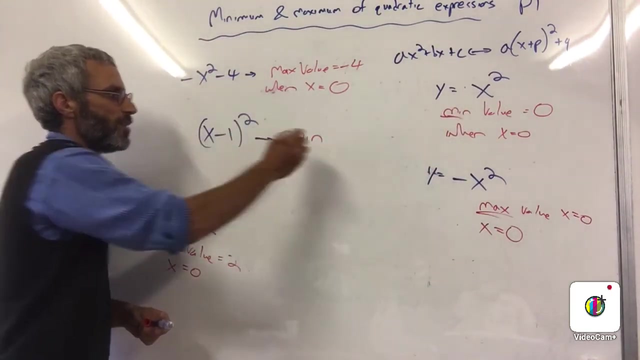 But the smallest it can be. what is the smallest that this can be? One. What's the smallest It's still can be? I mean, the smallest that this could be is zero. right, zero square is zero. So the smallest this could be still zero. The minimum value, the. 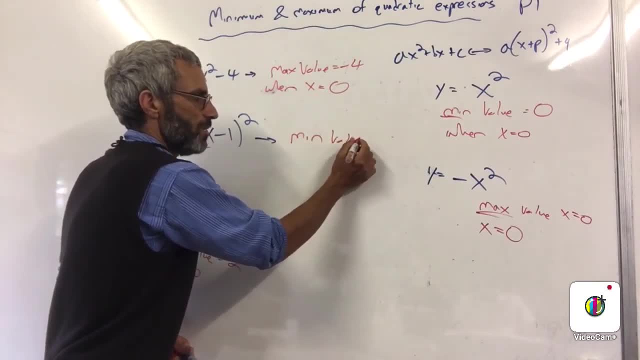 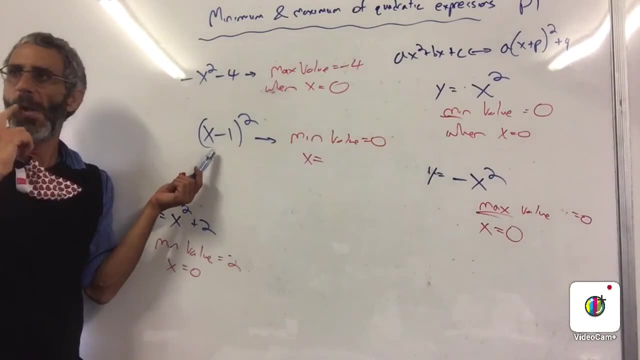 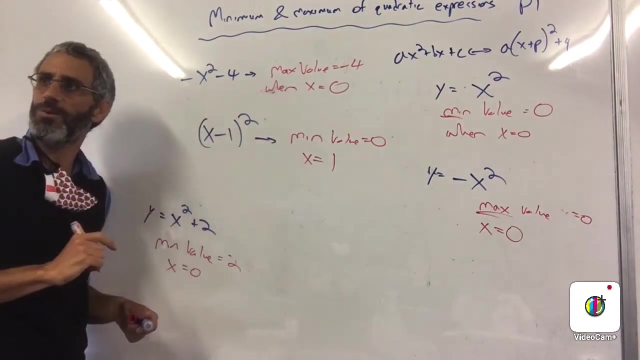 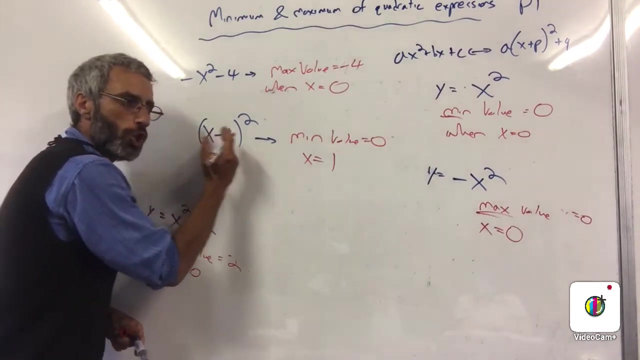 minimum value is still going to be zero. Minimum value equals zero, But what should x be equal to give zero? When x equals one, one minus one square is zero, Okay. Later, when we learn about function, we say there is a horizontal shift, Everything's moved to the right. This: 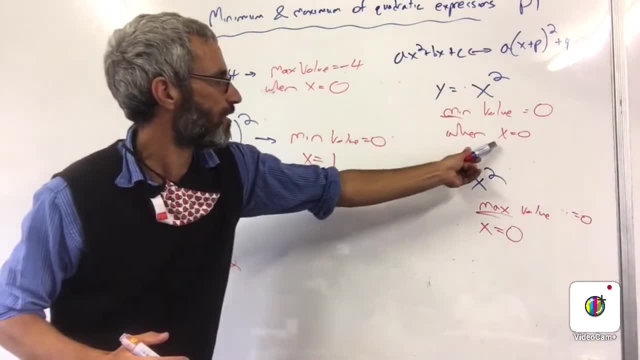 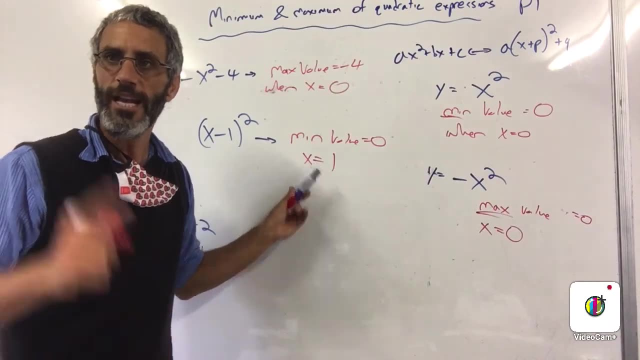 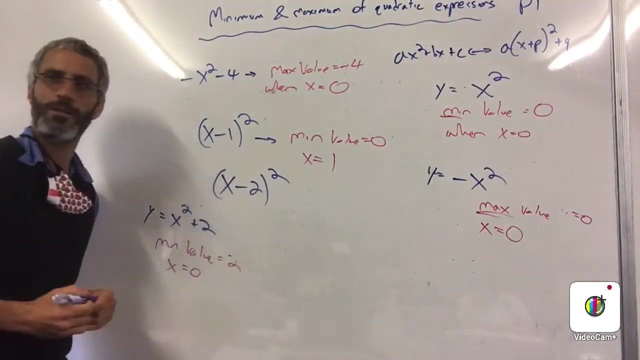 is the same as that. It's just now. the x was zero to give the minimum value. It's the same minimum value, but now it's when x is one. Okay, Let's do one more example, then I'll take a question. Let's say I have x minus two squared. Okay, What will be the okay? 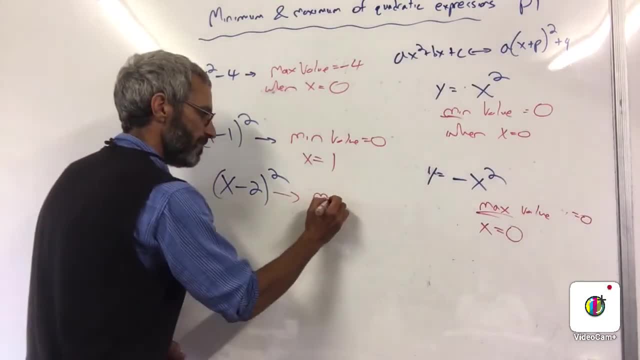 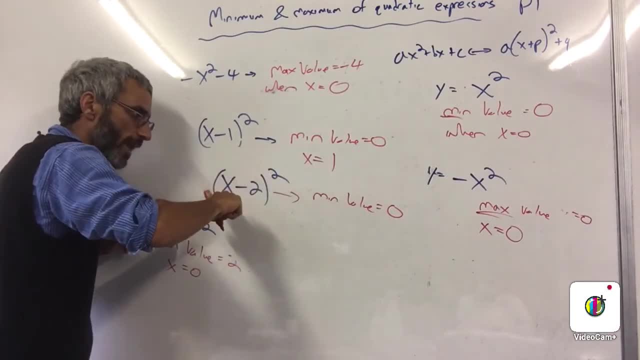 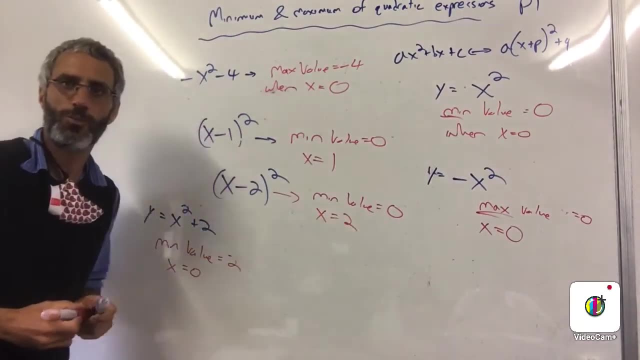 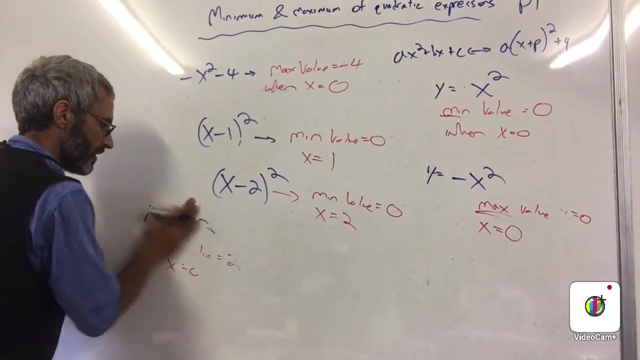 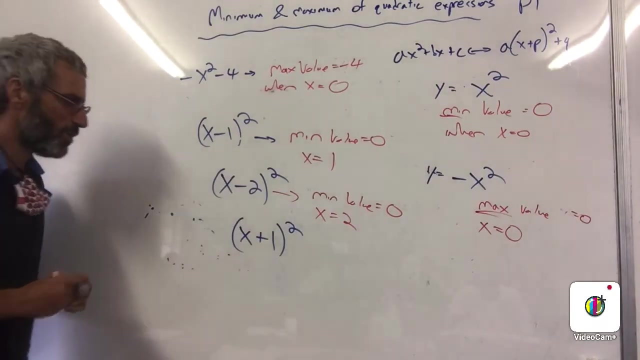 is a positive number. The lowest that it can be is zero. Okay, For which x will it be Two? x equals two. I'll just pose. it was a question. Great, Okay, so now. okay, let's do one more. That's going to be a bit confusing. What about x plus one squared? Okay, All right. 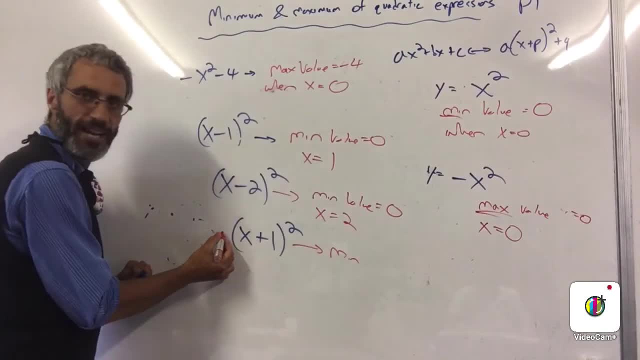 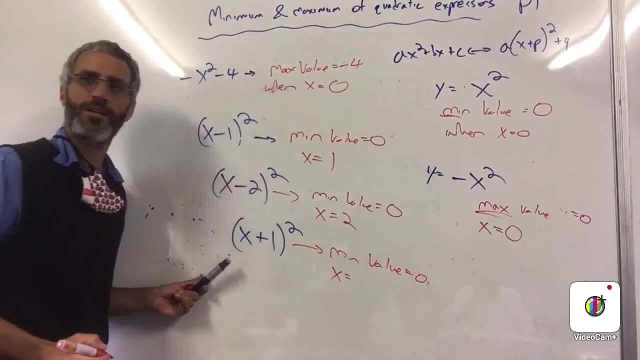 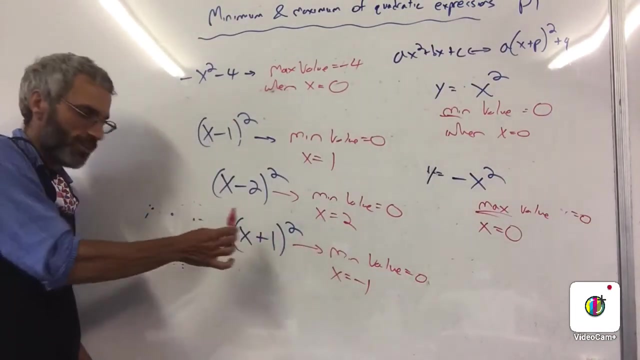 First, it is still a minimum, because I don't have a negative here. Minimum value is equal to zero. For which x is it going to be Minus one, Minus one. So now I have a horizontal shift. we'll call it later on to the left. 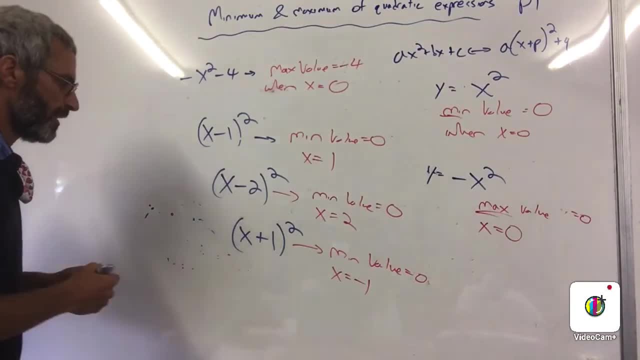 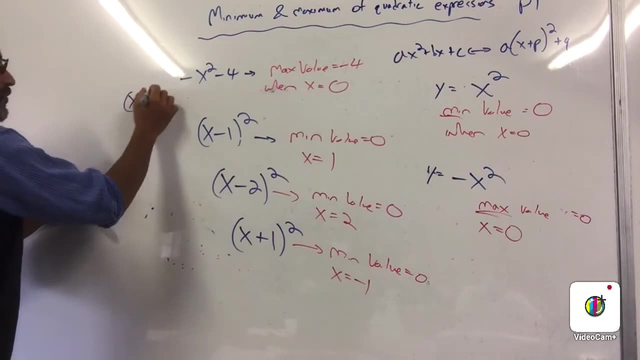 Okay, that seems to be alright. You're still fine with that. Let's do one more. Okay, let's take that one. One x minus one squared. but now we slap minus here. So what do we have now? Minimum or maximum? 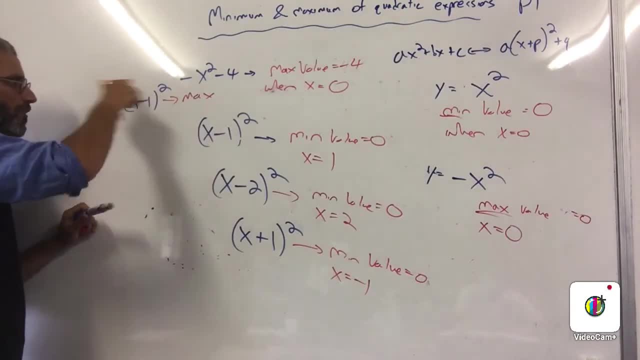 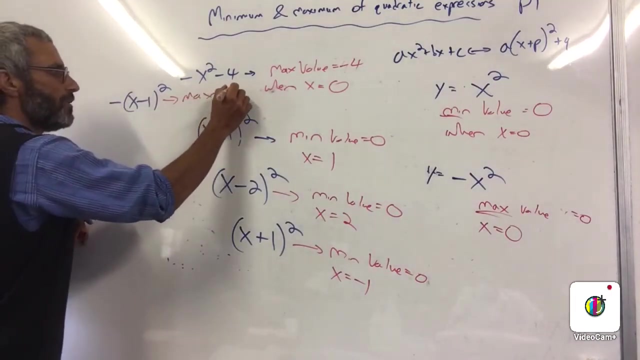 Maximum, Maximum. Why? Because this whole thing is positive, But now, with the minus, this whole thing is negative. Okay, So what's the highest? that a negative number could be Zero. Okay, So the maximum value? Oops, Equals. 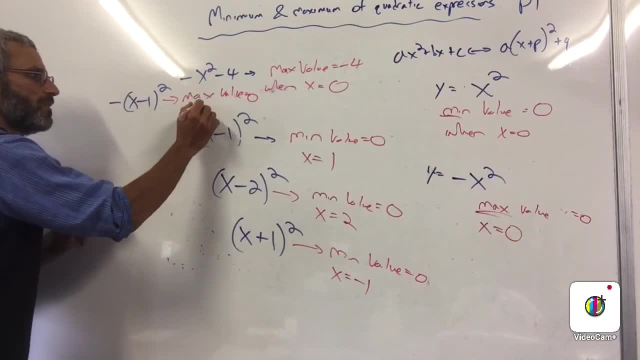 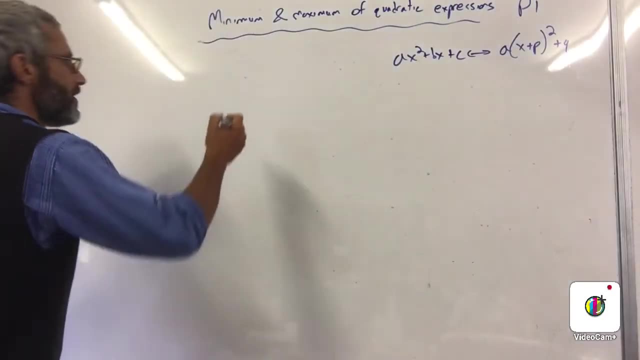 It's still equal to zero. For which x is it going to be? One Seems like you're getting it. Okay, let me just pause here, So let's do another one: x plus two, put a minus squared. 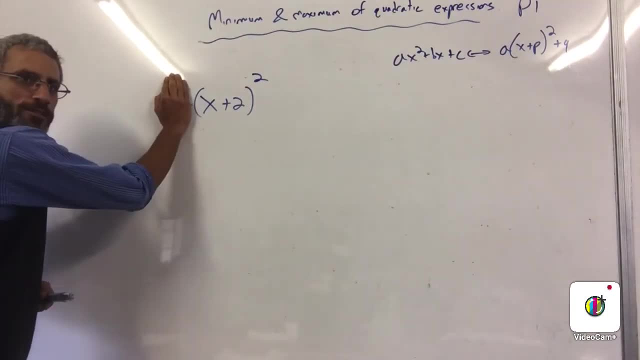 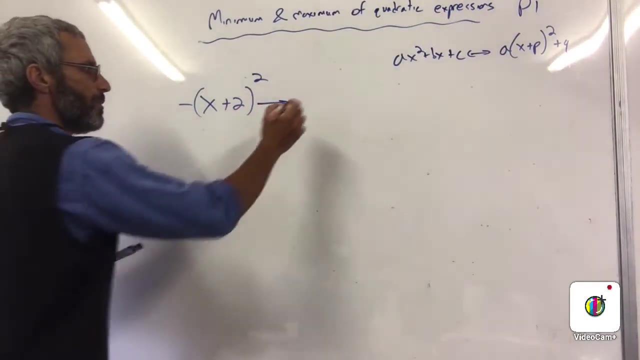 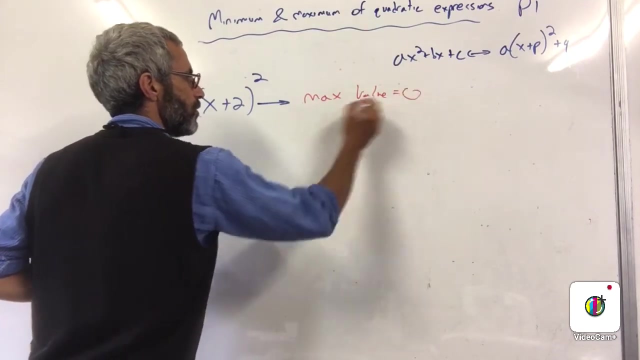 Okay, Remembering this is always positive, That means when the minus is always negative, That means we're going to have a maximum or minimum. There will be a maximum value which is equal to zero, And that happens when x equals negative two. 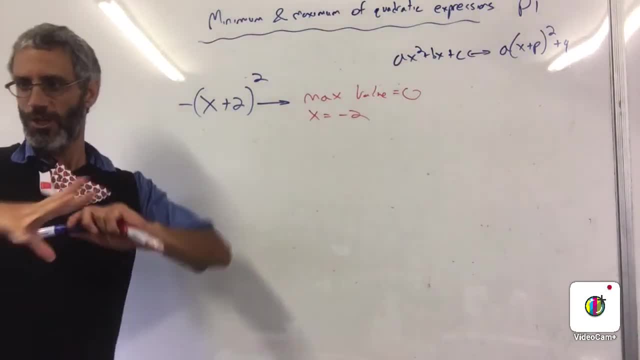 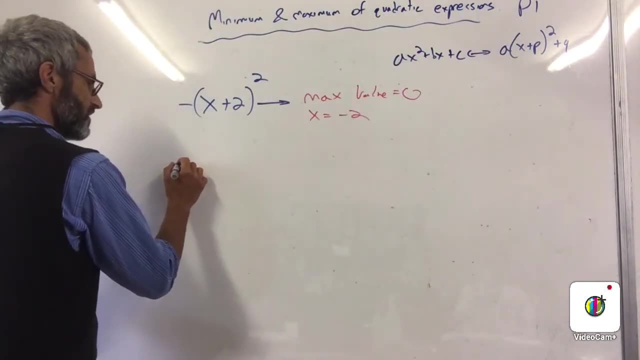 This is not difficult for you. Okay, now we're moving to the last, most general case, Most general case. Okay now. yeah, Let's do like this. Actually, let's put it this way: If I had minus two here, or let's do another number. 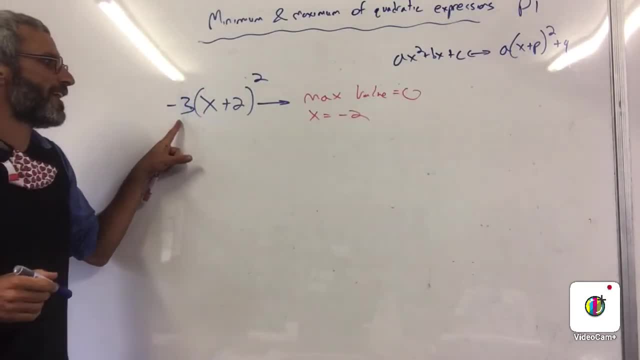 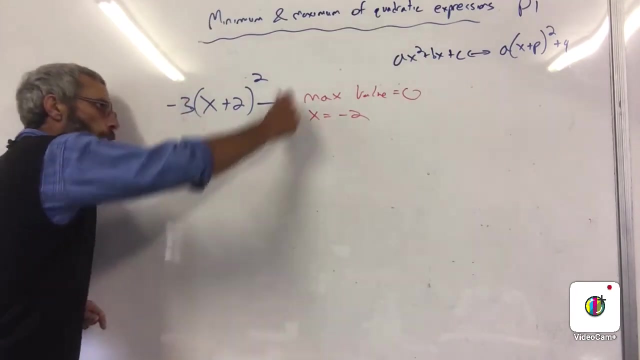 Minus three. Is it going to affect anything here? No, It's still minus two. So what I'm saying is: this is still negative. This whole thing is negative. Therefore, there will be a maximum value. The maximum value is going to happen when x is minus two. 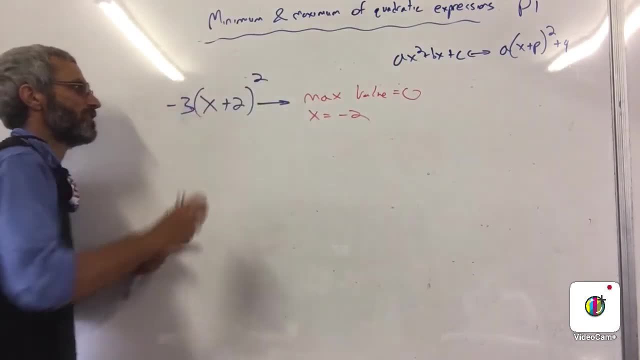 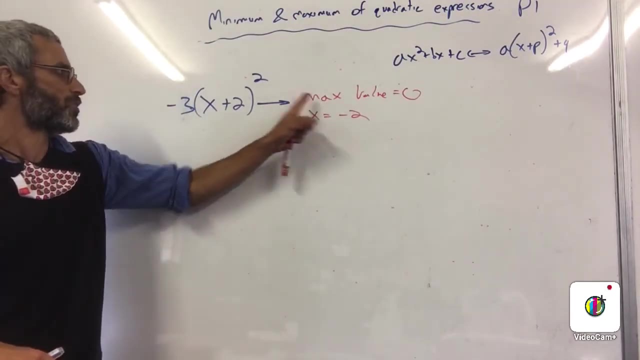 Because then it becomes zero And zero squared is zero, And zero to minus three is minus three. So we still have the same answer. Is that right? Okay, it's still going to have a maximum value which is equal to zero. 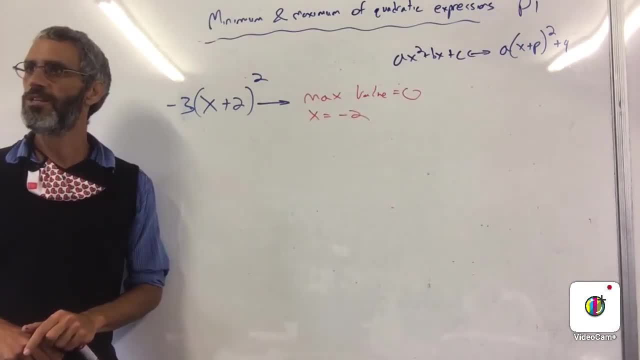 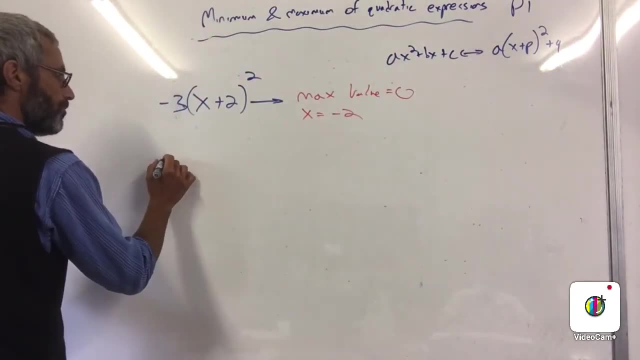 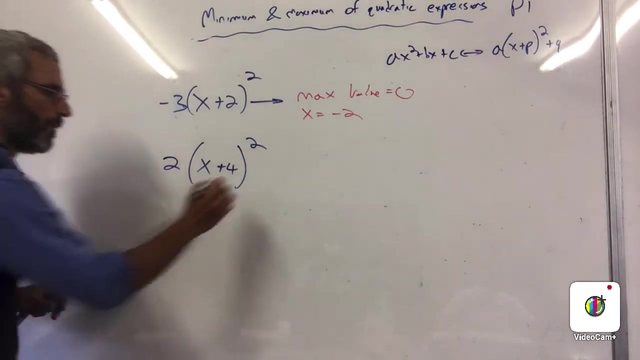 And it happens at x minus two. No, I'll just pause there. It's a question mark. Let's do something else now. So let's say we'll put two x plus four squared Plus three. Okay, Right, first of all, 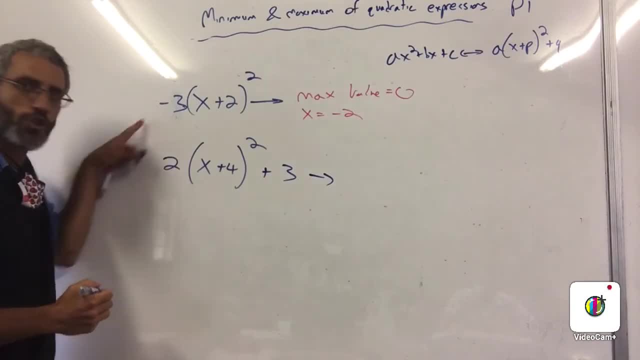 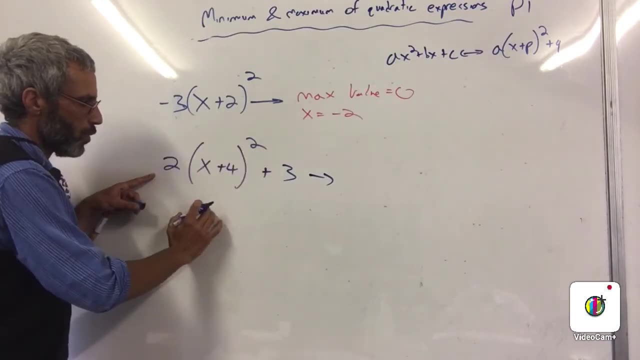 Maximum or minimum. It's minimum Because this is positive here. Okay, This is always going to be positive number. Okay, So it's just going to get bigger and bigger and bigger. As I get x, it will get bigger and bigger and bigger. 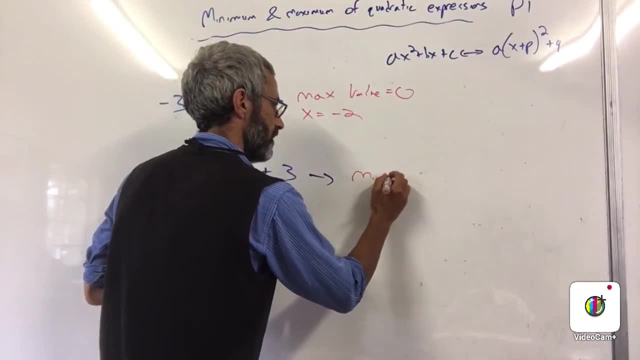 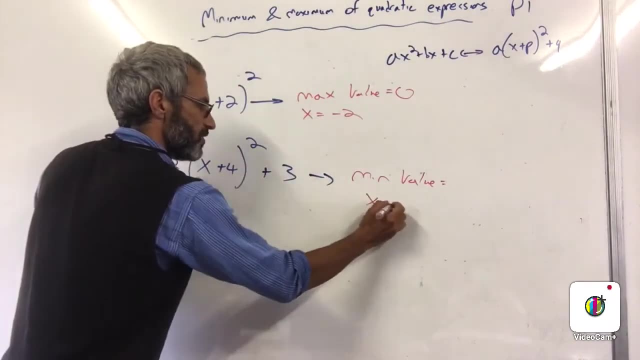 But that means there is a minimum Right Minimum value. I'm not going to write what the minimum value is there yet. For which x is it going to be minimum? When is the minimum going to be? When x is equal to? 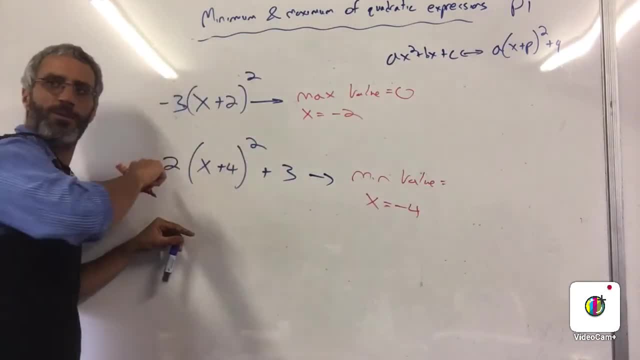 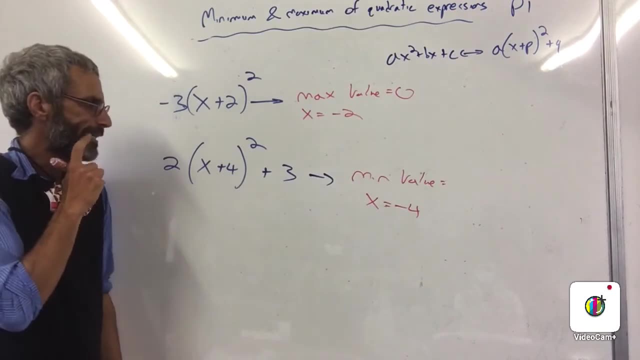 Negative four. Negative four, Because when that's negative, Negative four. This thing is zero. Okay, What is the minimum value? now, Minus three. Say how much. Minus three, Minus three, Plus three, Plus three. 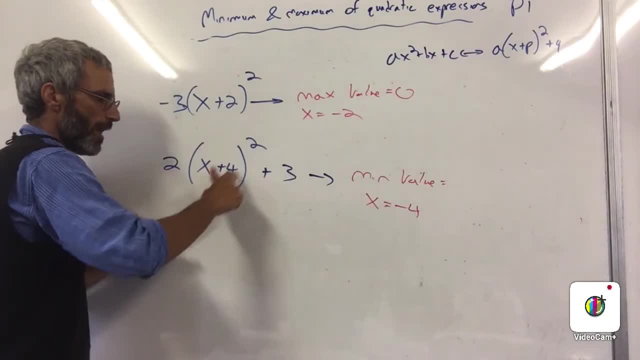 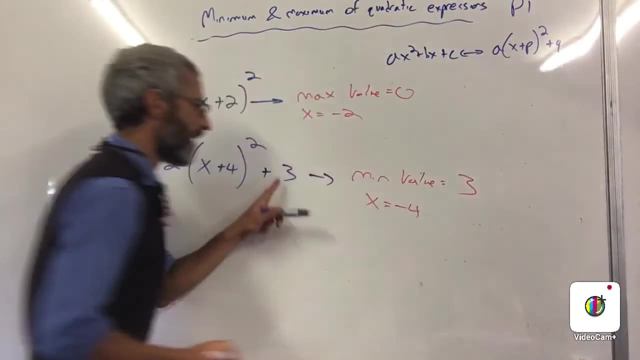 Okay, When x equal minus four, Minus four plus four is zero. So zero squared is zero. All this is zero Plus three. So the minimum value now moved up. All my minimum value were zeros here because I didn't have plus something. 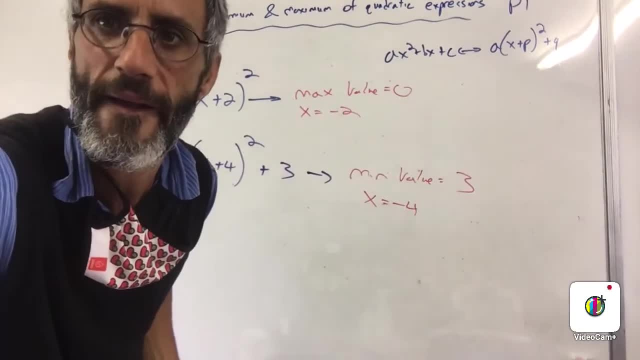 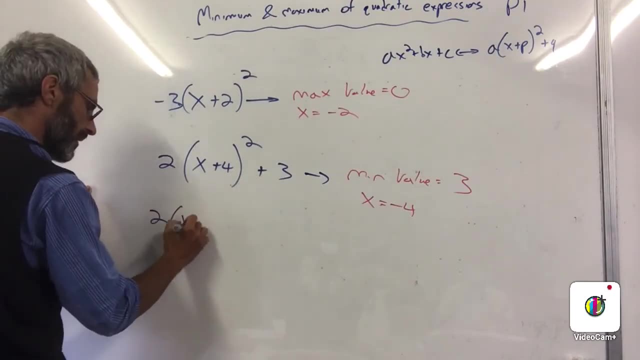 Now it's moved up, So let's go with. I don't know what do you do? you want the same thing, but just, instead of that, minus three, okay. So two x plus four squared minus three, Okay. 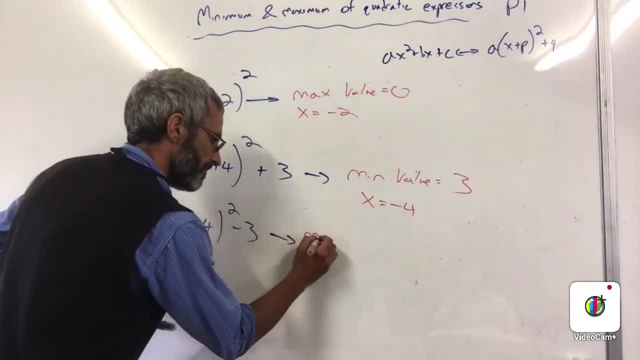 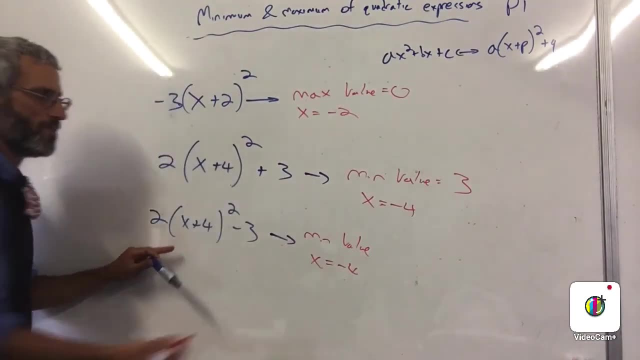 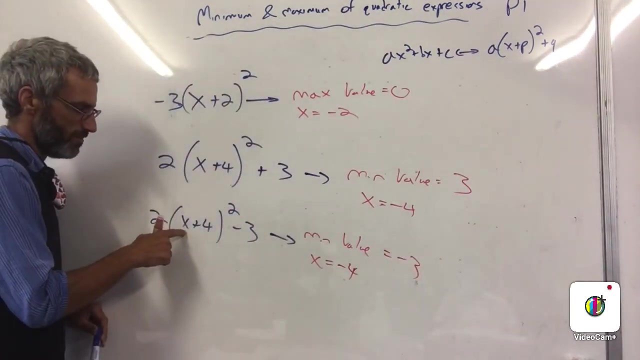 First of all, minimum or maximum Minimum. Still minimum value: Okay, X equal negative four. And what will be the minimum value? Minus three, Minus three, Yeah, Because when that's x minus, When that's minus four, this is zero. 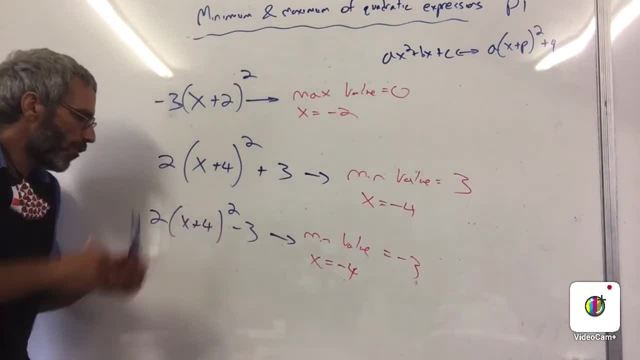 This is zero. End up with minus three- Another way of thinking about it. Look This whole thing, the square. that means it's always positive. The lowest it can be is zero. So this whole thing, the lowest it can be is zero. 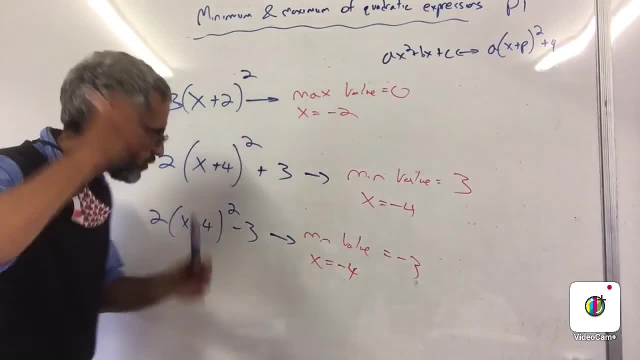 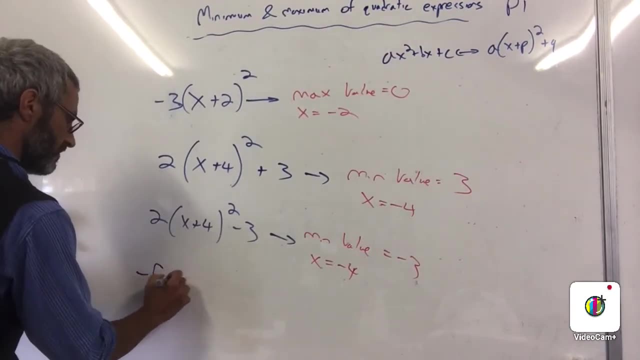 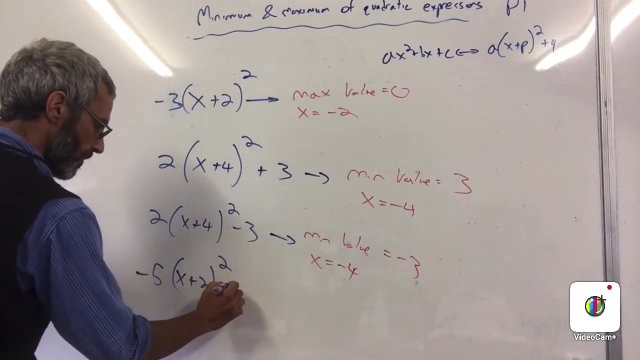 So zero minus three is minus three. Okay, Let's do one last one and then you're ready on your. you're ready, So let's just put some minuses, Okay. So minus five, X plus two- squared- I don't know what- plus one. 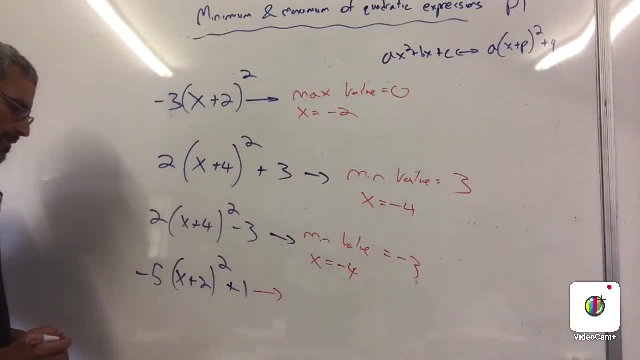 Okay, What would that be? Okay, So it will be a maximum because this whole thing is negative. Okay, And that maximum value will be- let's try straight away, I've heard the right answer- One When this is zero, that will be one. 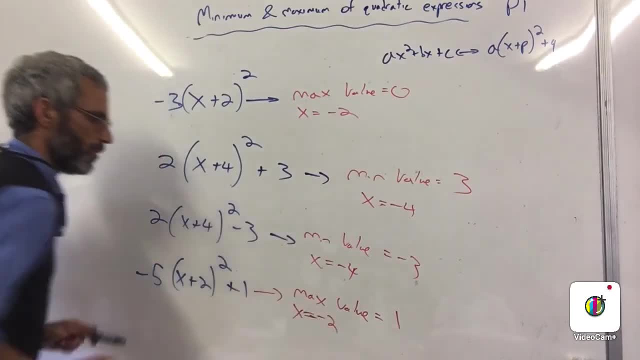 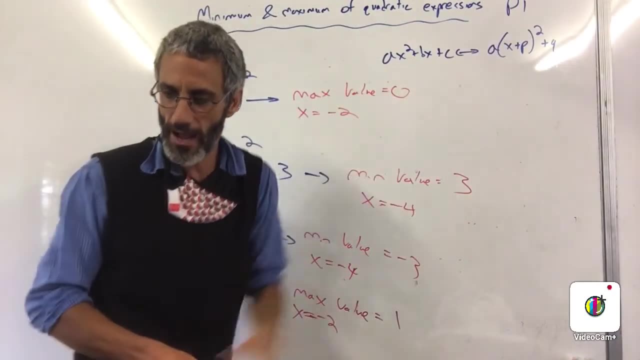 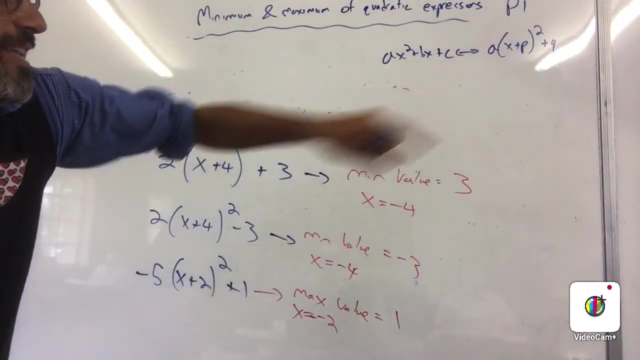 And x must be equal. Negative two, Negative two. And now, guys, I'm ready to tell you why we actually done that, Okay, Why we done that. Okay. If I have, I don't know what, Let's take, let's take this one. 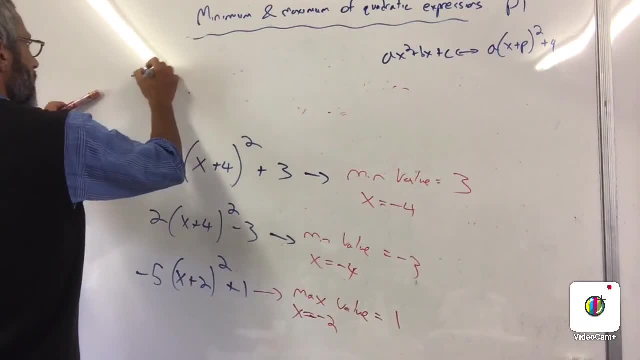 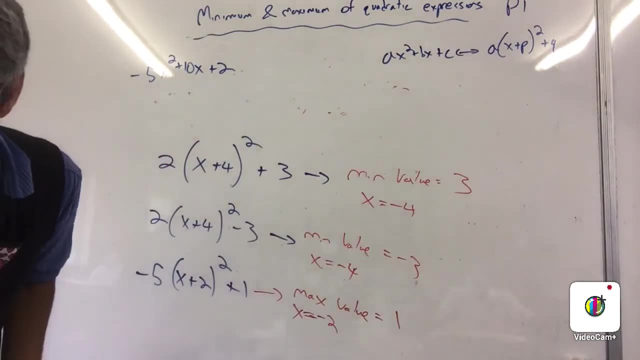 Okay, Earlier Finn, you asked me to do that. Minus five x squared, plus ten x plus two, If I give you this quadratic expression, can you tell me if it has a minimum or maximum? In fact, you can. You can tell me it's a minimum or maximum.